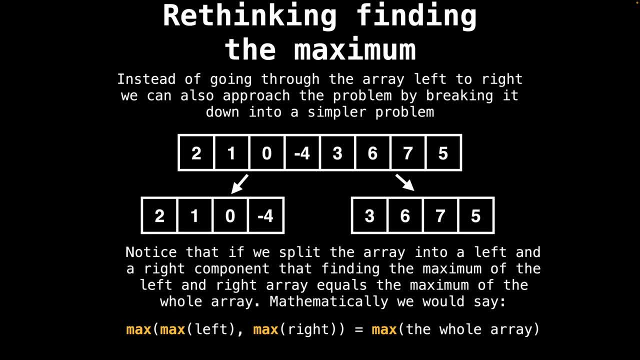 the array into a left and a right component that finding the maximum of the left and the right array equals the maximum of the whole array. This is important to note because it means that splitting up the array to find the maximum will not change the value of the true maximum of the whole array After we split the original. 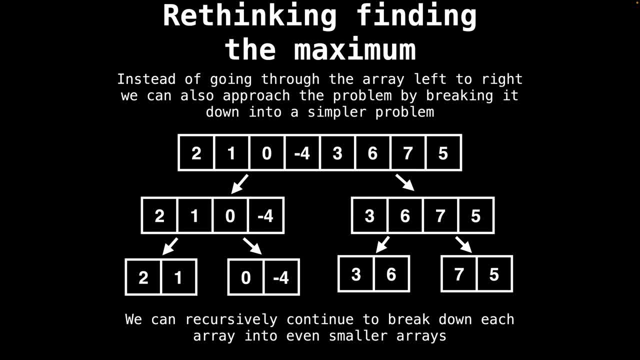 list into two parts. we can further split the lists again into four lists and then split those four lists into eight lists composed of individual elements. Now, going back to the original problem we're trying to solve, which is finding the maximum element we know. 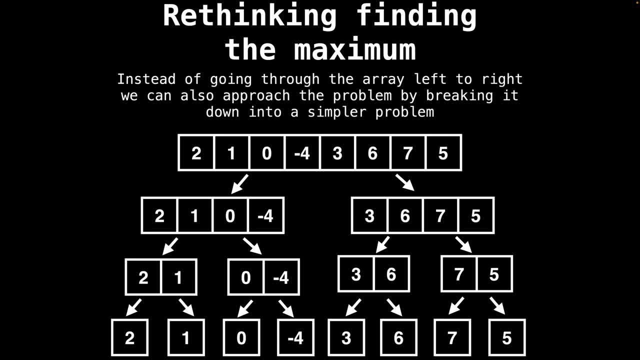 that we need to combine two lists of numbers together to find the maximum of those two lists. We also trivially know that the maximum element in a list with a single value is the value itself. With this information, we can begin finding the maximum value of the entire. 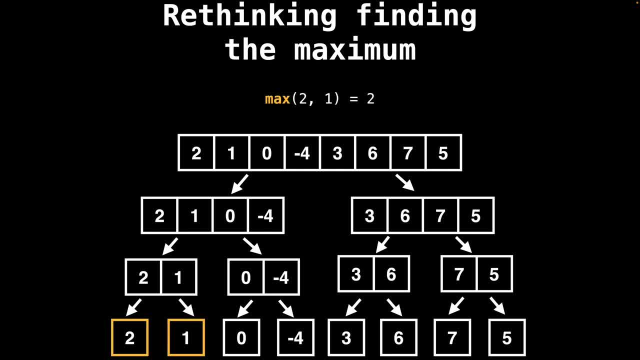 list by working our way upwards. Let's begin combining lists together on the lower left, starting with two and one. The max of two and one is two, So we can return to and one is two, And then we can return two and one is one, And then we can return two and one is. 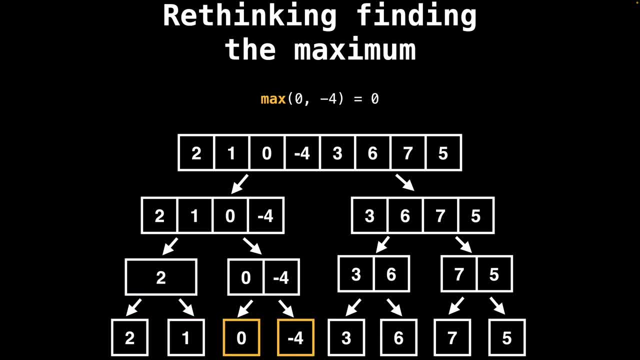 as the maximum value. then we take the max of zero and negative four, which is zero, then the max of three and six and seven and five. After that we can reapply the same process to the third row. the max of two and zero is two, So we place two as the maximum. 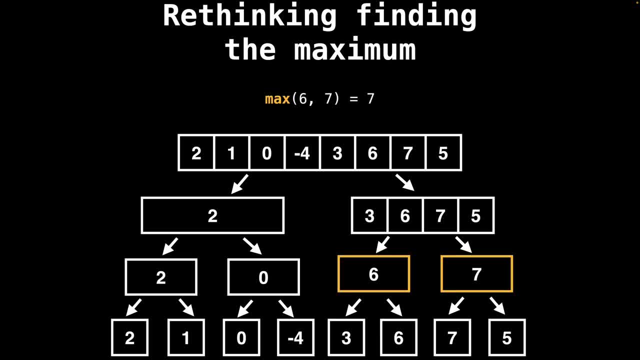 value for that sub list, And then the max of six and seven is seven. So seven becomes the max value of the right sub list. Then we reapply the same process for the final two sub lists. the max of two and seven is seven And in the end seven is the maximum. 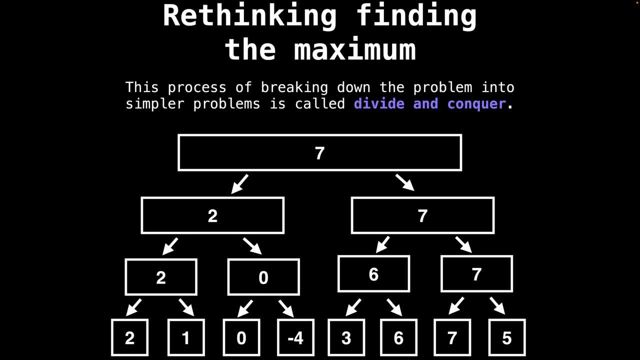 element in the list. This process that we just saw- breaking down a problem into simpler sub problems And then solving those sub problems- is what we call divide and conquer. Okay, awesome. Now let's take a glance at how the divide and conquer algorithm for finding the 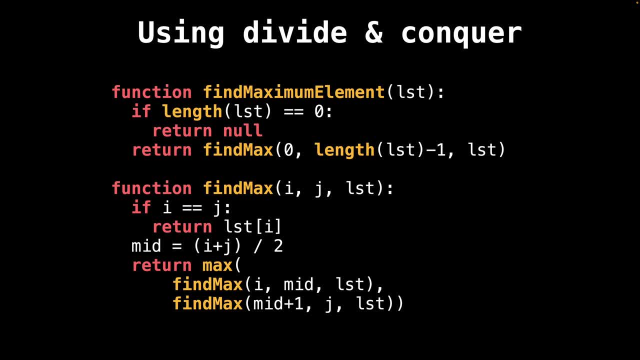 maximum element is implemented, You'll see that we're repeatedly splitting the current segment based on the interval from i to j at some midpoint. However, before we run through this code in detail, I want to illustrate how the division of the segments takes place. 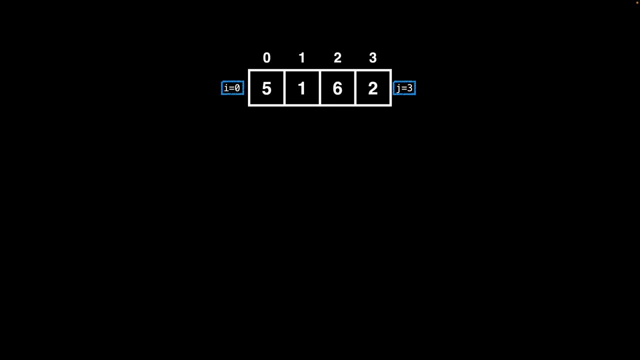 because it might not be so obvious. Let's imagine we have a given segment and we have a given list And our objective is to divide it into smaller lists. To accomplish this, we maintain a record of the indices representing the segments of the list as we progress down. 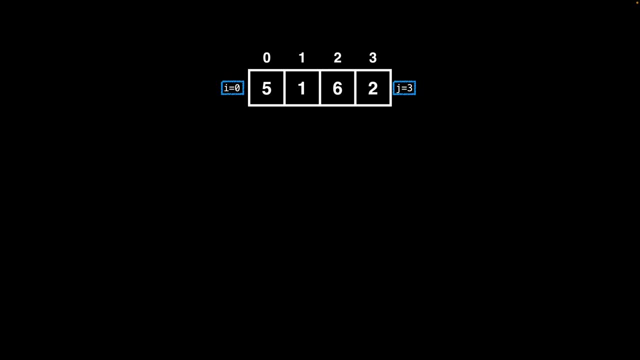 the tree. This approach enables us to keep track of the specific portions of the list that we're working on, eliminating the need to create a copy of the segment itself. So highlighted in blue are the indices representing the initial segment. I represents the left index of the segment and the index of the second segment represents the index of the segment. 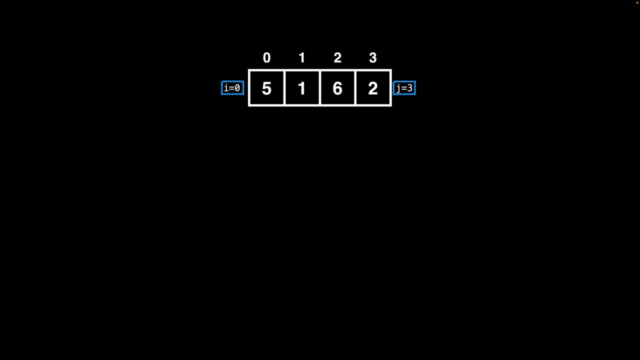 And j represents the right index of the segment. When splitting the segment zero to three, we find the midpoint by adding indices i and j and dividing the sum by two. the midpoint position allows us to compute the new indices for the left and the right segments In the 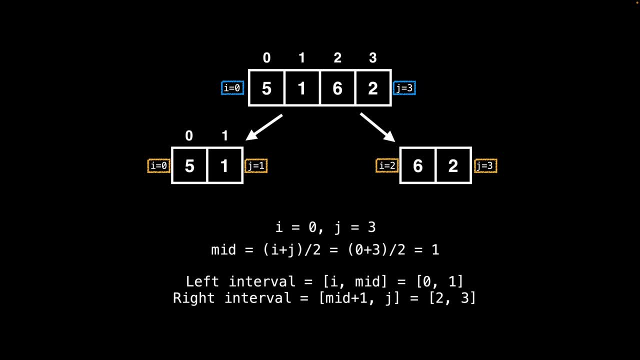 given scenario, the midpoint is at index one, resulting in the left segment being zero to one and the right segment being two to three. We can reapply the same process to split the left segment again. In this case, the midpoint is at index zero and the new left segment is at 00.. And the right segment between one. 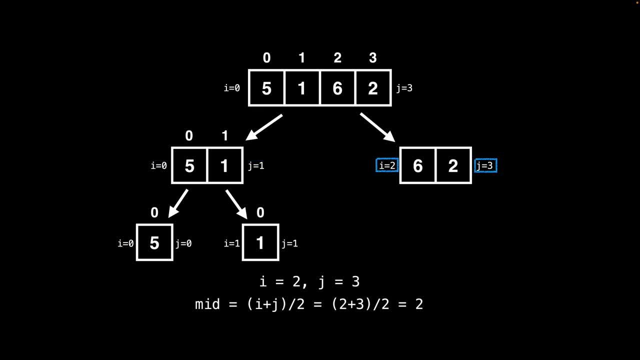 and one, both inclusive And similarly for the right segment. here the interval two to three gets broken down into a left segment of two comma two And the right segment of three to three, And that's how the splitting process works. 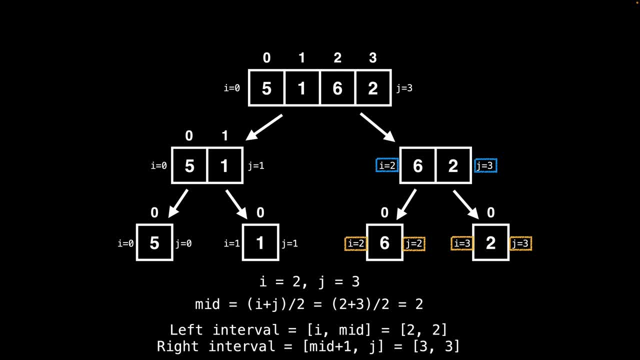 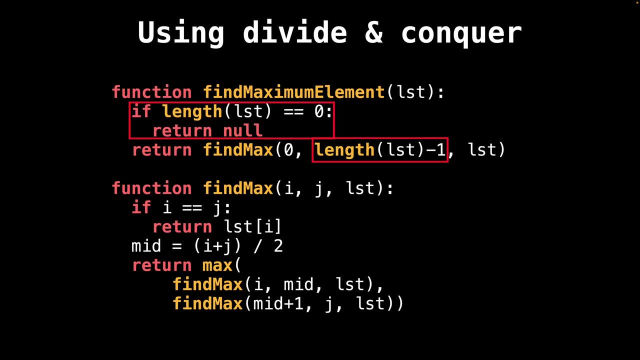 in a nutshell Now let's go back to the pseudo code for a moment Now. looking at the code again, you can see that inside the find maximum element function, the first thing we do is check if the list is empty and return null if there are no elements. The reason for doing. 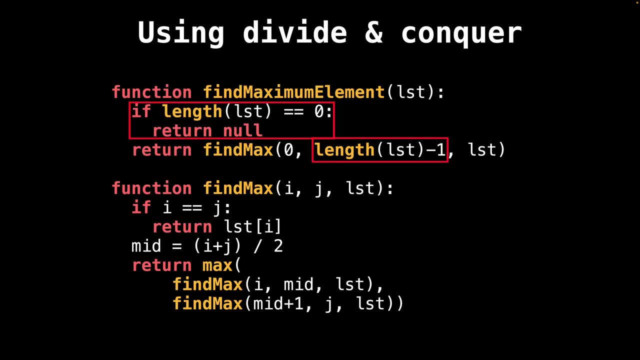 this is that there's no way to divide up an empty array any further, So immediately handle this edge case. It also prevents us from having an empty array. If we take this edge case, negative index value on the next line, which would cause the recursion to spiral into a. 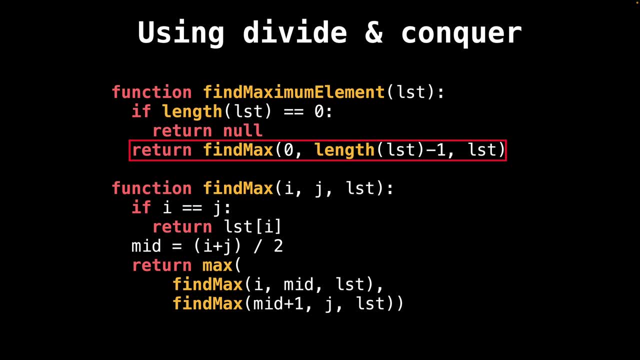 stack overflow error. On the next line you can see that we're calling the find max function below, which is what actually finds the maximum. the input to this function takes two indices, i and j, which represent the segment of the array which we want to find the maximum for. 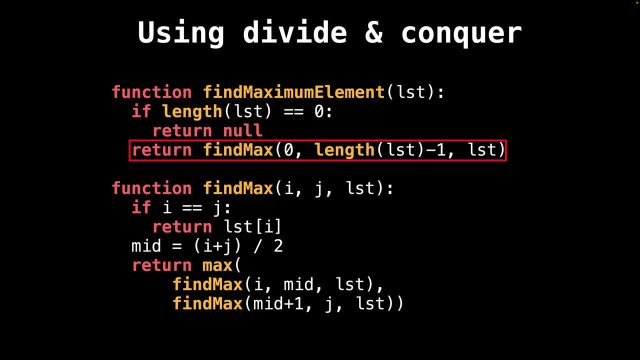 index. i is the left endpoint and j is the right endpoint. Since we want to find the maximum of the whole array, we pass an: i equals zero as the left most index and j equals the length of the array minus one as the right most index. Now let's take a look at what 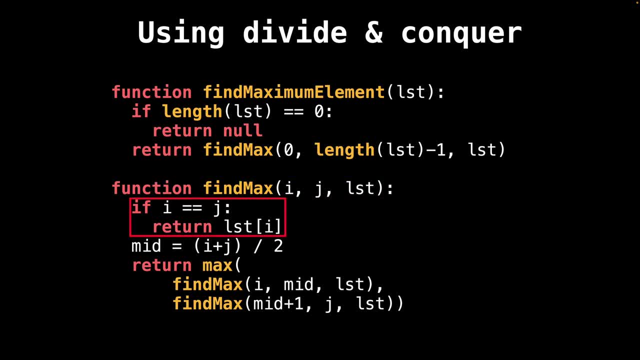 exactly is happening inside the find max function? The first thing we do is check if i is equal to j, which means that the size of the segment or interval is a single element. Since we know that the maximum value for a single element is the element itself, we simply return the. 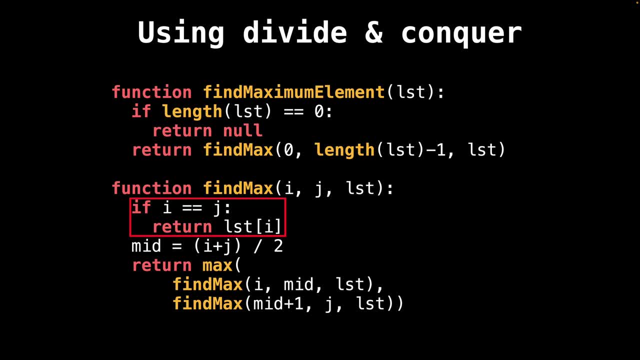 element at that index, And this constitutes our base case. Next, in order to split the segment in half, we need to find the middle index position between i and j. This allows us to split the current segment into two parts: a left segment from i to the midpoint, and. 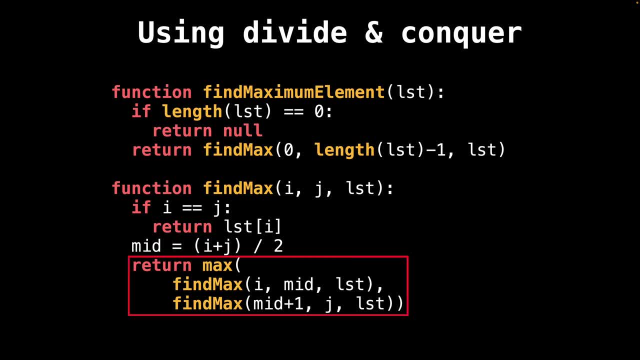 a right segment from the midpoint to j, Then on the next line you can see that this is where we do both the segment split And then the combination of segments. on the callback, The first to find max function call corresponds to the left segment and the second call to the right segment, Since the indices 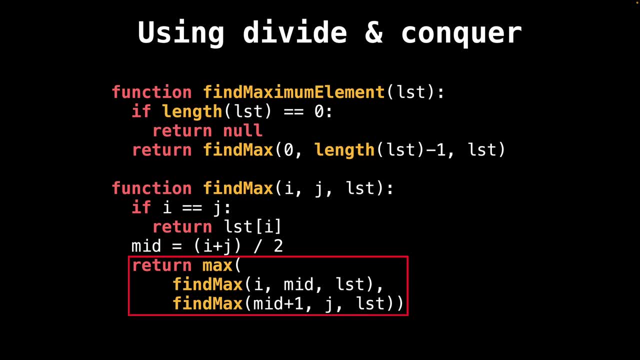 for the segments is inclusive. the left segment ranges i to mid. but to avoid an overlap, the right segment starts at mid plus one and ends at j, And that's how you use divide and conquer to find the maximum element in the list. 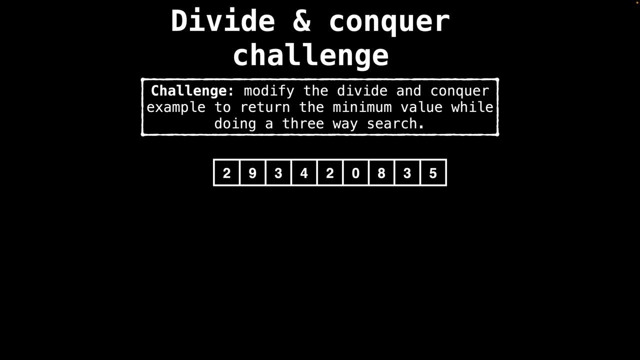 Alright, so we just finished taking a look at how to use divide and conquer to find the maximum element in the list. The strategy we looked at repeatedly divided the segments into two parts. For this challenge, I want you guys to modify the previous code example to return. 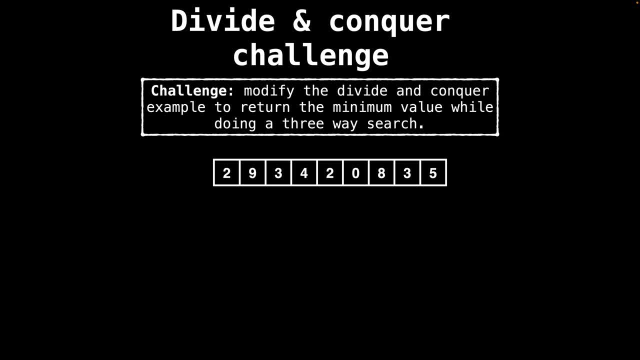 the minimum value in the list while doing a three way search instead of a two way search. For example, in the list here, we divide the nine elements into three segments of length 30. And then we further divide up those segments to three more segments of length one each. 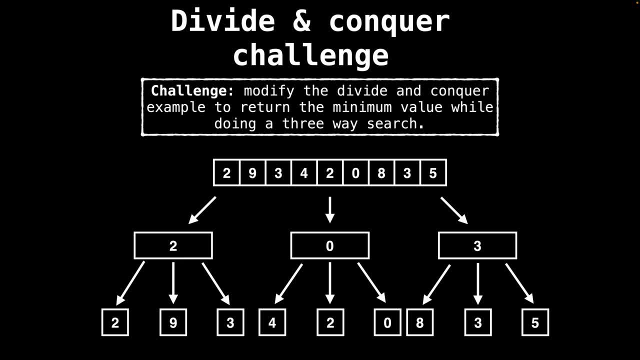 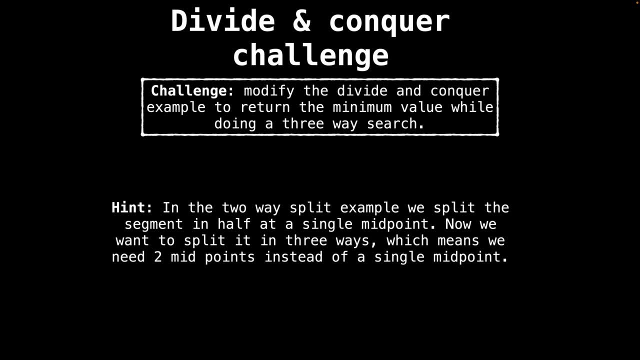 We can then find the minimum value of the whole list based on the method of splitting, the same way we did previously. So before you guys go ahead and try and implement this, I want to give you all a hint. In the two way split example, we split the segment in: 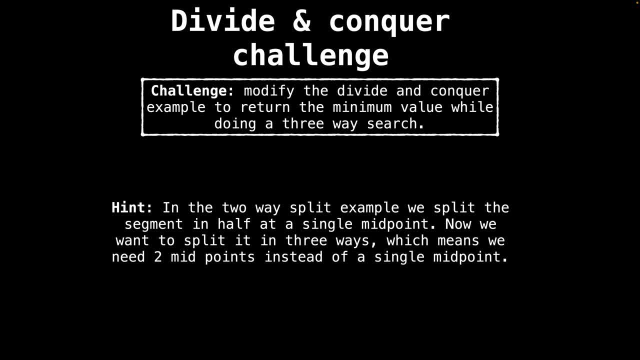 half based on a single midpoint. Now we want to split the segment into three parts, which means that we will need two midpoints instead of a single midpoint. Alright, I'm going to give you guys a moment to pause the video, if you want to give us. 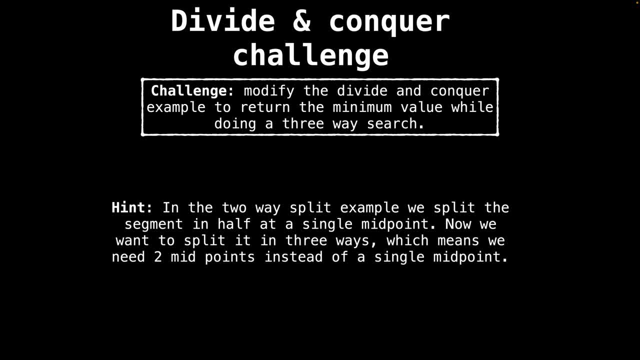 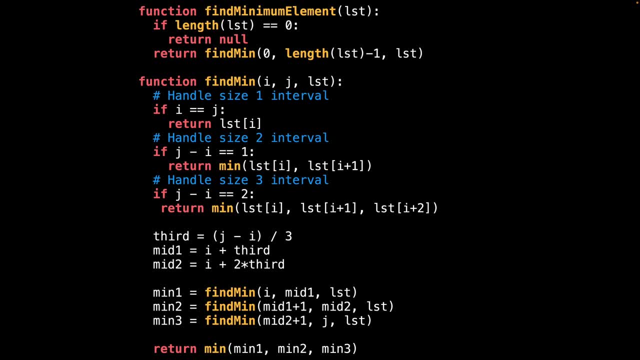 a try. I'm going to reveal the solution in the next slide. Awesome, I hope you guys were able to give that a try. And here's one way to implement the three way split using divide and conquer strategy we just talked about. So, rather than 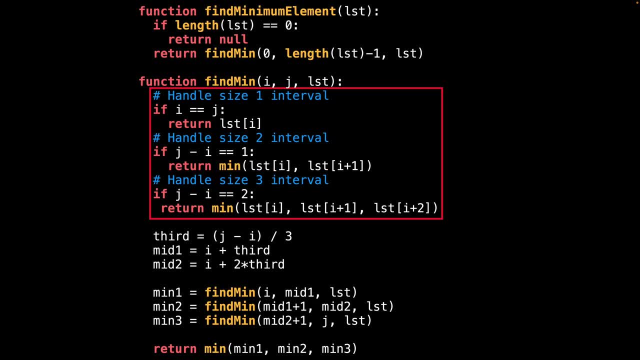 having a single base case. I address three different base cases, when the size of the interval is three or smaller, And these cases simply return the minimum of the existing values. This approach simplifies handling the scenarios where the interval consists of precisely three elements or cannot be divided any further. If none of these base cases are 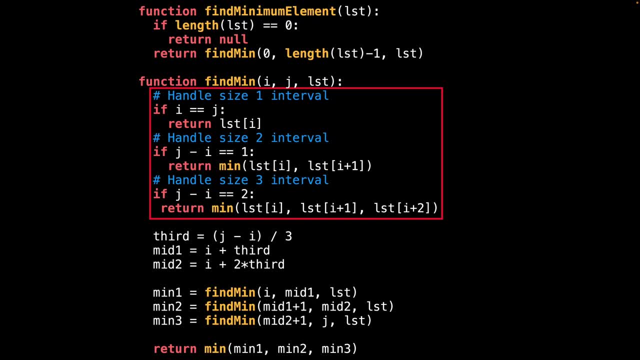 encountered. we know that our interval comprises of four or more elements, So we're going to split the interval into three segments. When the interval is four or more elements, we can split the current interval into three segments, Since we want three separate segments. 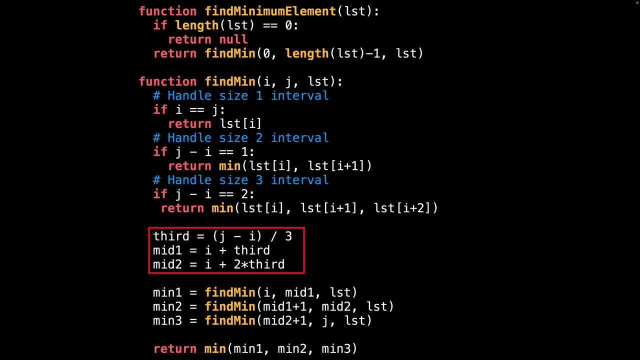 there has to be two different midpoints by which we can split across. These midpoints can be found at the one third mark and at the two thirds mark. Once we have our midpoints, we can then split the current segment into roughly equal thirds and return the minimum.